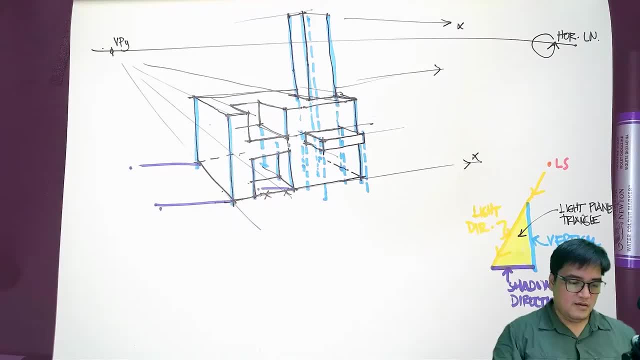 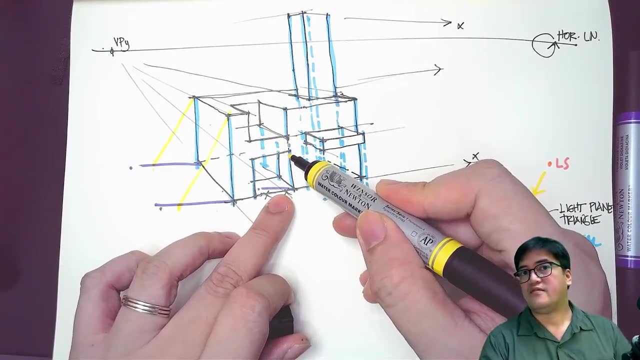 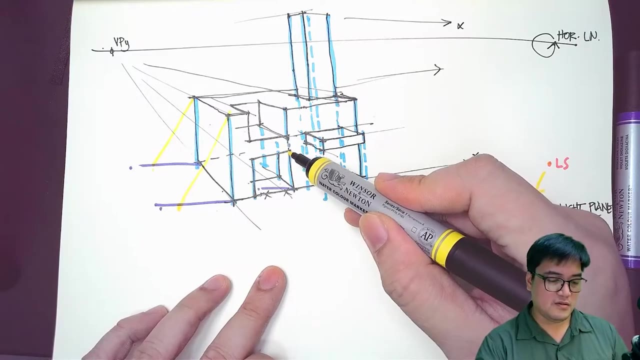 So we can see that the plane is coming from or distant lighting is coming from. So let's determine that to be like something like 60 degrees, Like this edge here. it stops here, on the top most of this opening. I'm going to replicate that same angle over to here. Just make sure that they're 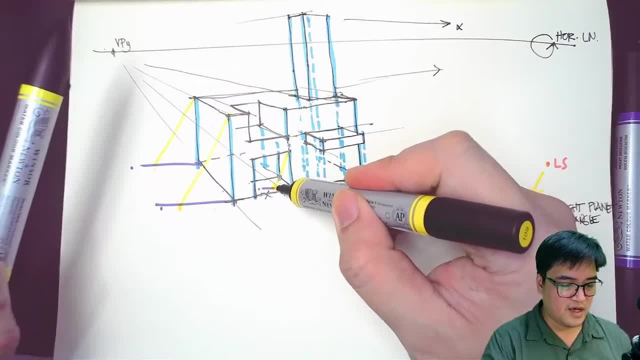 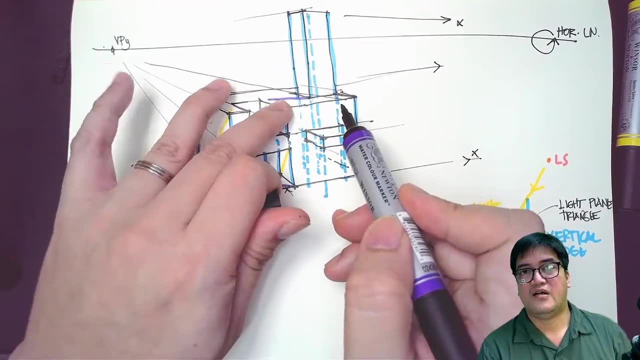 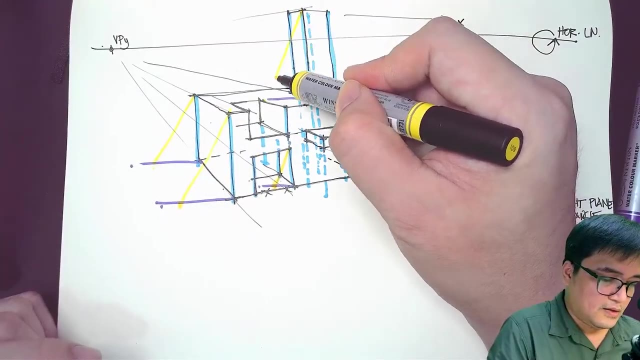 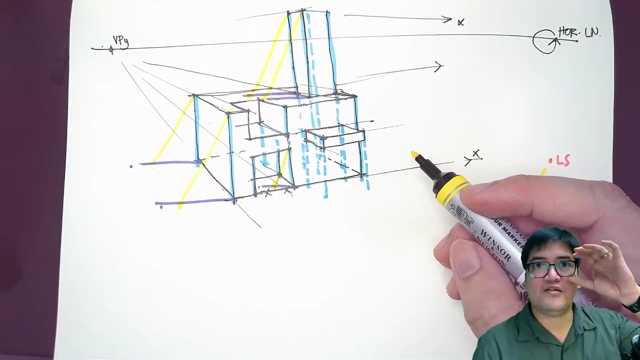 parallel. You can use a pen like so and try to determine that same angle. So this is the plane of the ground, It's on this plane of this object itself, And plot this same angle here. All these light direction lines are parallel to each other. 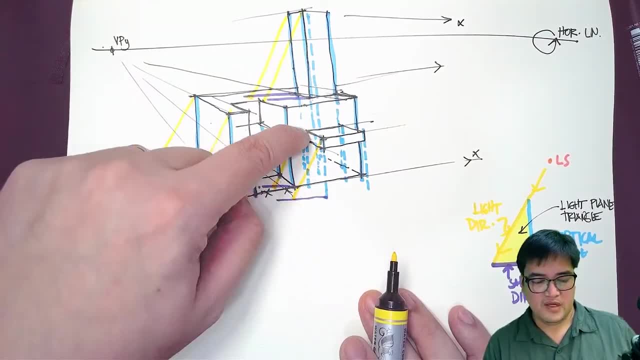 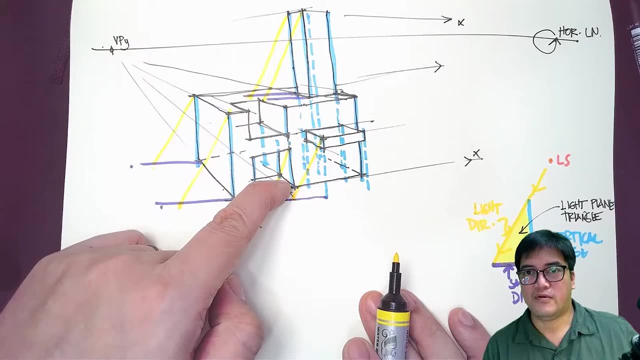 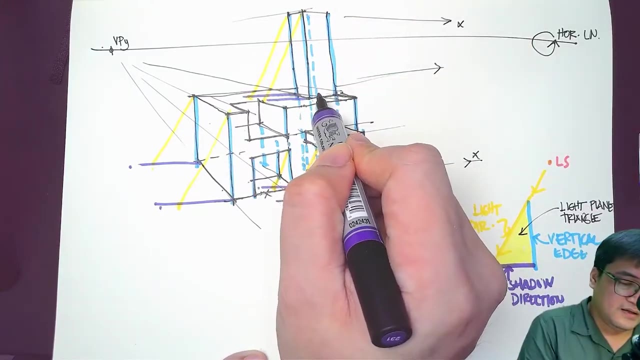 Later we'll come back to this, because if we imagine this, Okay, so this is our vertical line and the shadow line is going to go into the building. So I need another shadow line on for this vertical edge behind. So first determine where it's originating, which is there? 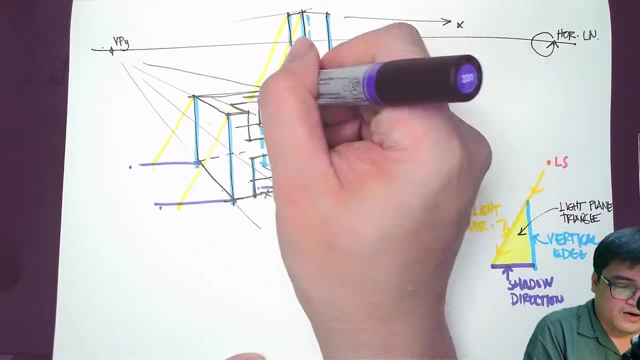 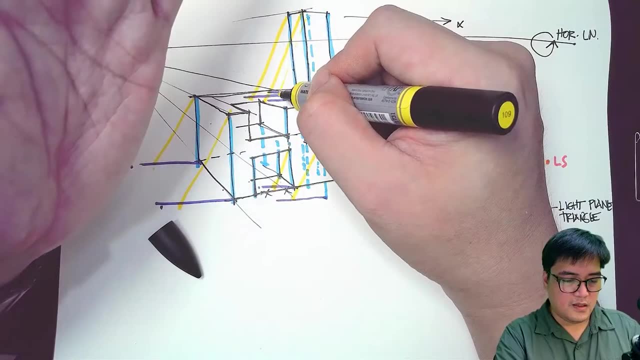 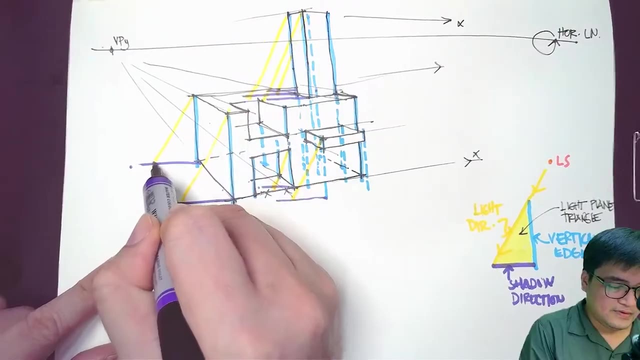 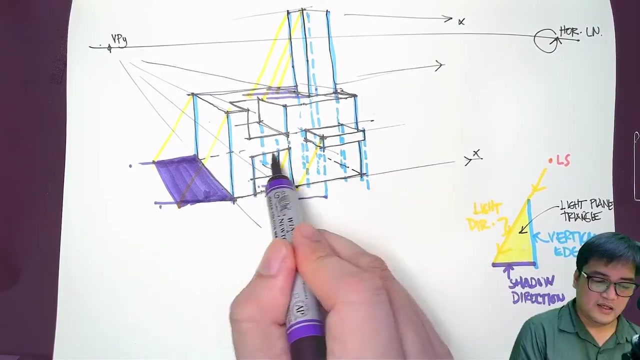 Right close to this and then draw a horizontal line parallel to the horizon line, You can determine the simple points that have to be drawn. So I'm going to use a line that is already established, Since I already determined where it intersects. This is along X. So therefore the line here. 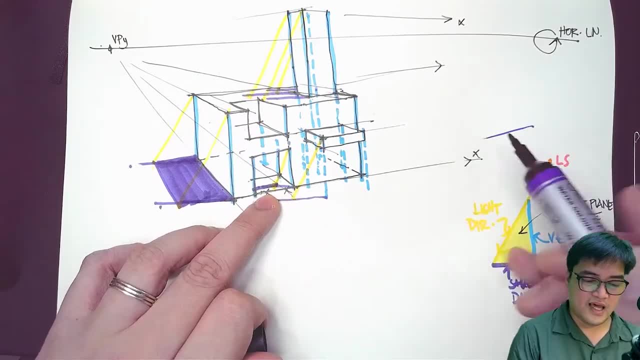 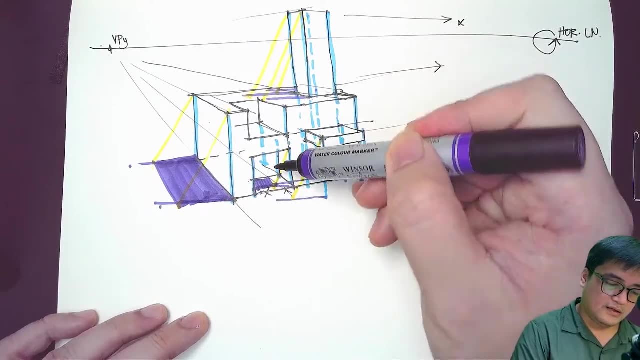 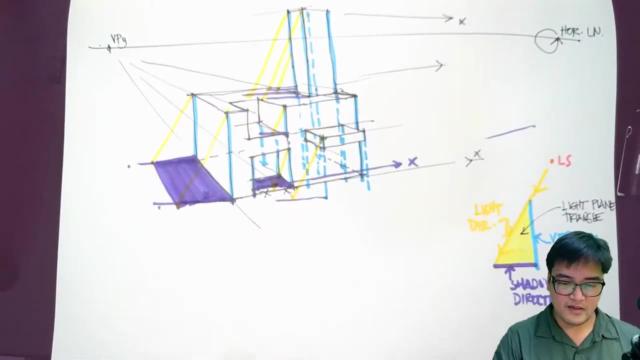 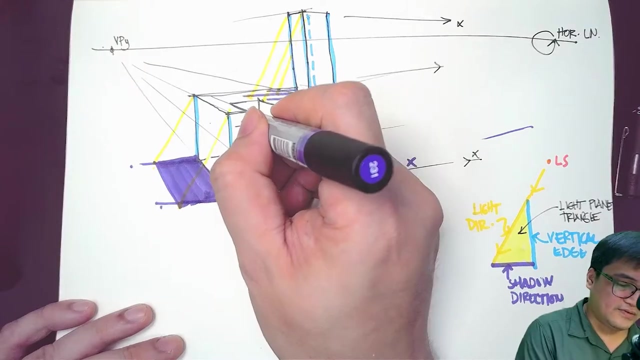 needs to be casted, The line needs to go towards X, and that creates the shadow cast for this one. Here you can do this, You can do this, but except that here's a complex complications here. Now this thing, the shadow line for this one, This vertical, is going in inside this solid object. 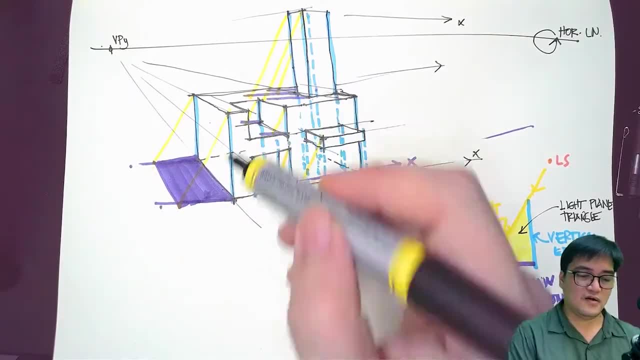 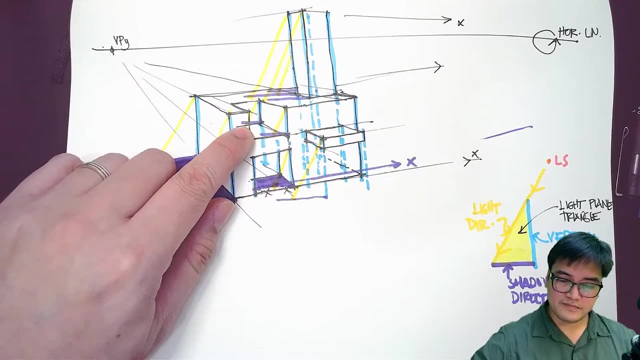 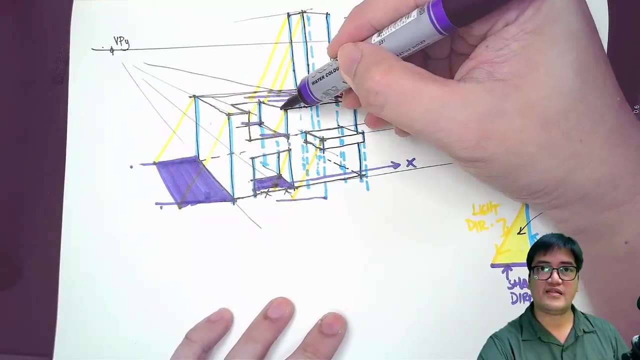 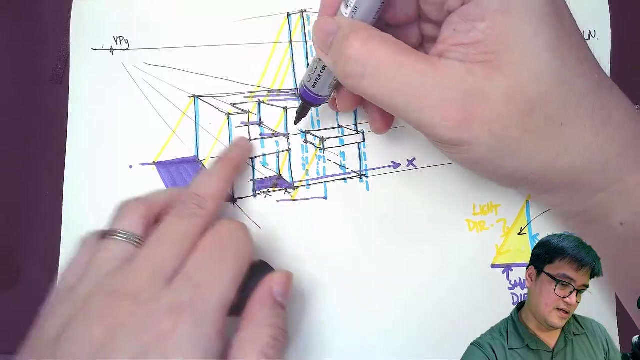 So the light source is light direction line is going inside the solid object. That gives me this information where whereby, since it's going in, Okay, so now I can cast the shadow casting for this edge starting from where it intersects with the. so I started with this and it goes towards vanishing point Y, it hits the. 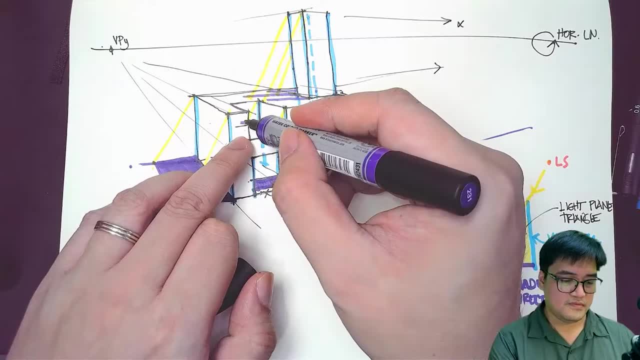 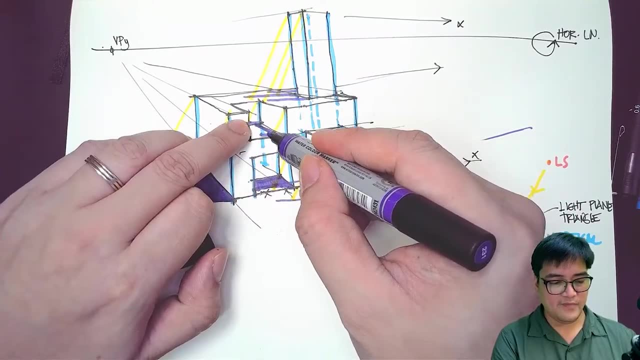 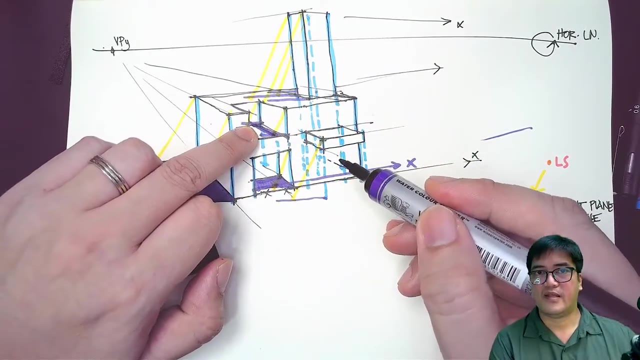 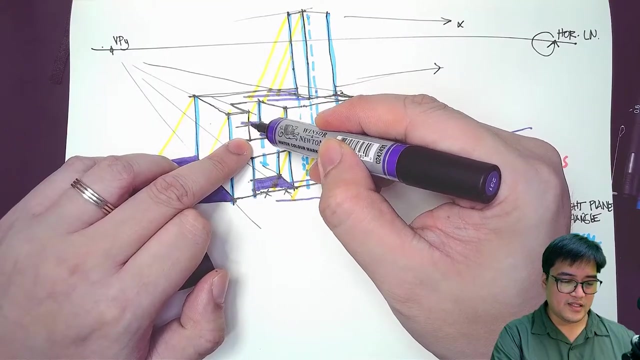 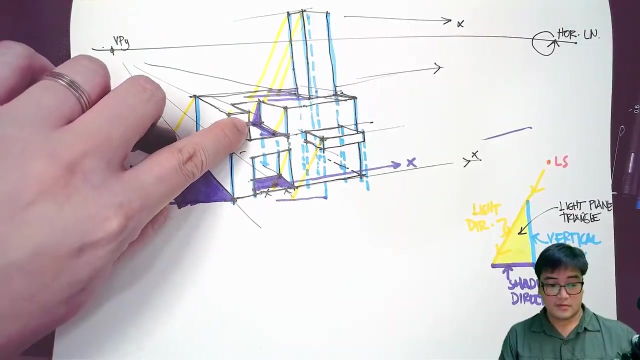 edge over here and this should connect this. so this point and that point should connect. and then, if it stops here, over to the this plane, vertical plane, and that determines now the shadow casting of for this, because it, since it hits this plane, it now creates the shadow on this plane. but if you notice that you 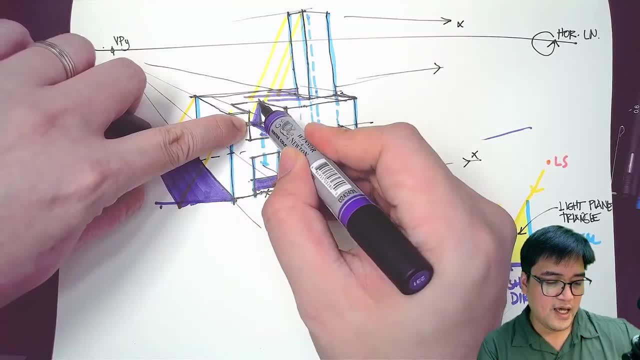 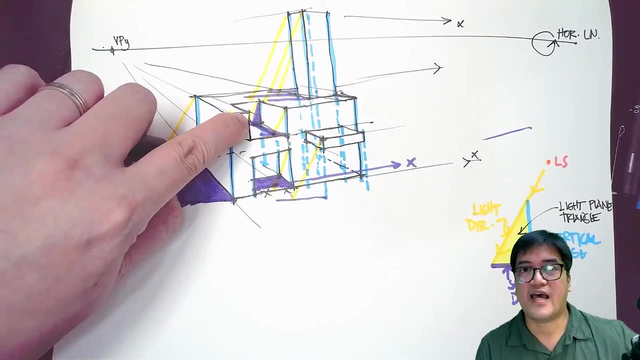 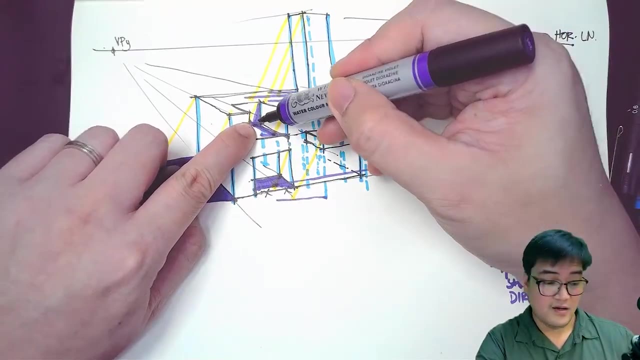 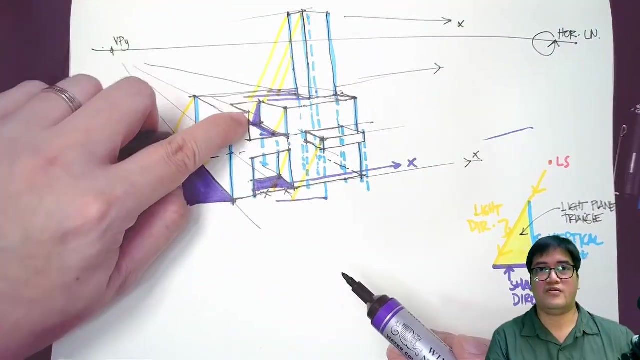 know what went on as the shadow line and the light direction line going inside. it's this point: if they intersect here inside, from this point, first point to that point, and then when it hits here on this edge, this corner, inch this plane and that plane. this is how you determine that vertical shadow casting. so it's. 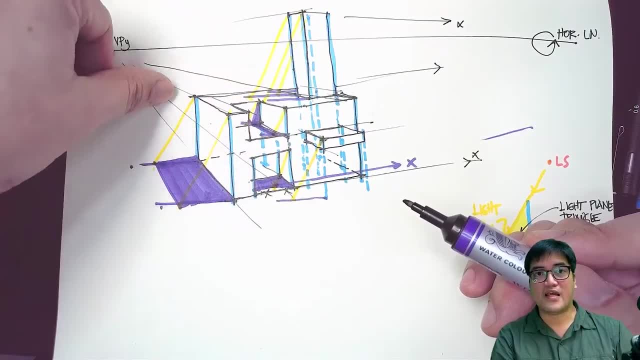 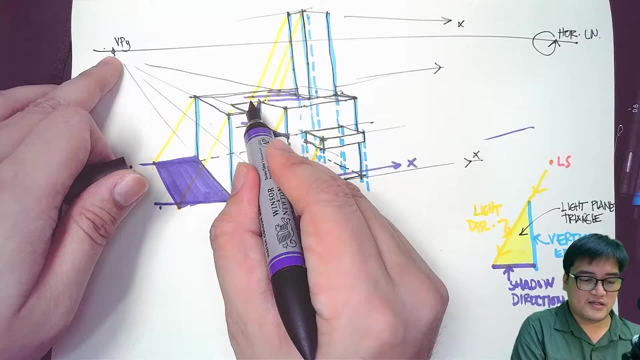 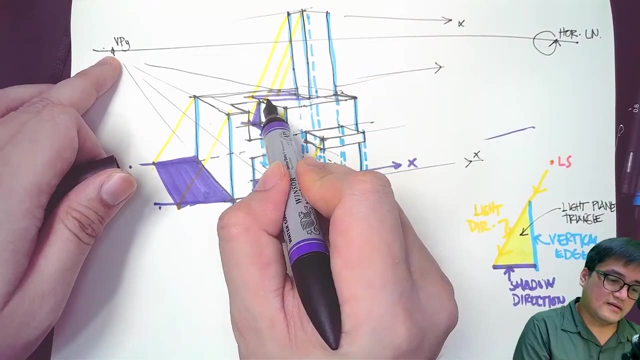 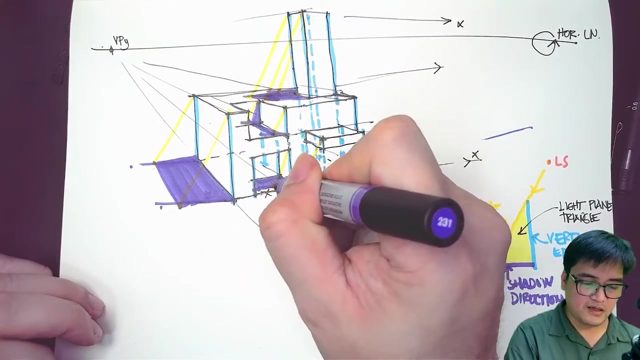 different. so this angle result: it's not the same as for this one. the shadow cast for this part is actually going to be here onto the surface, top surface of this first volume, so we still need to determine the shadow direction, which is this, and, of course, the light direction from the top of here, parallel. 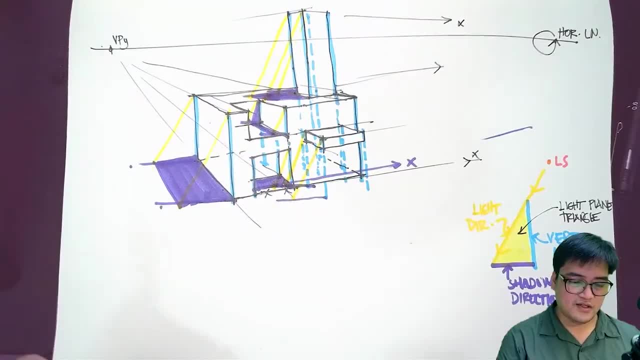 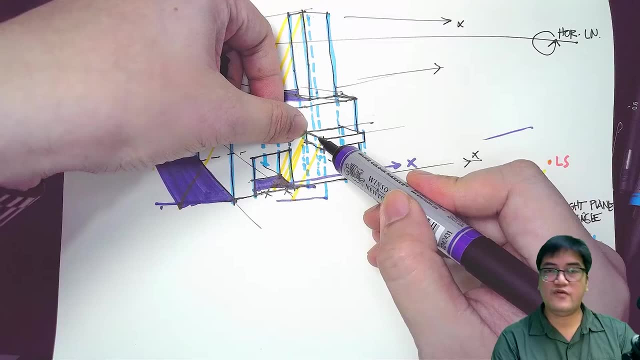 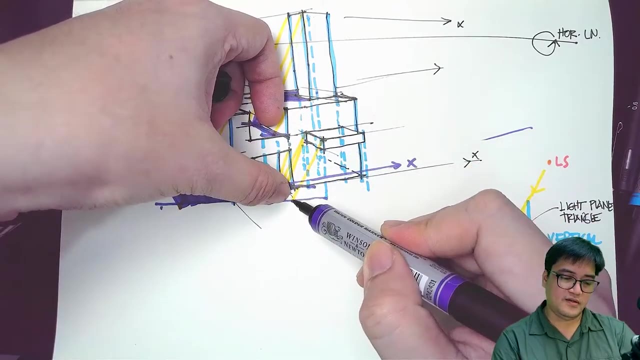 it's somewhere there inside, yeah, and that gives us context to where it's supposed, where it's supposed to go. I mean, where's the point of that? so the shadow edge for this one, at least initial part of this, is this point. is this point here? casted it to this point. 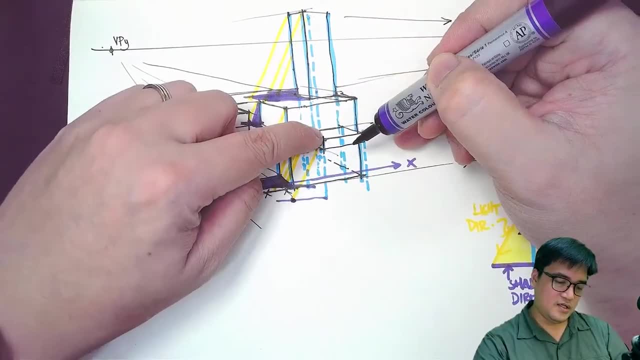 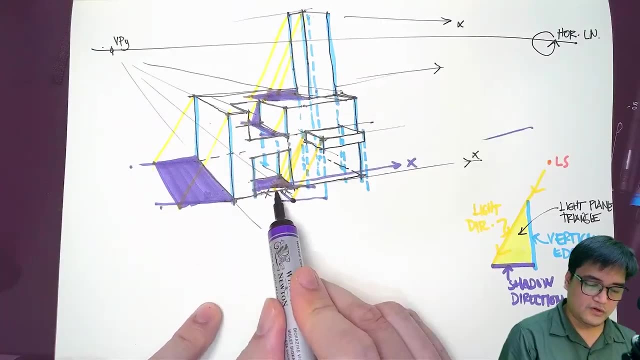 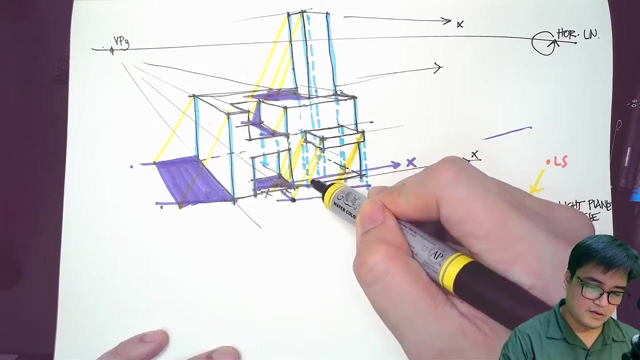 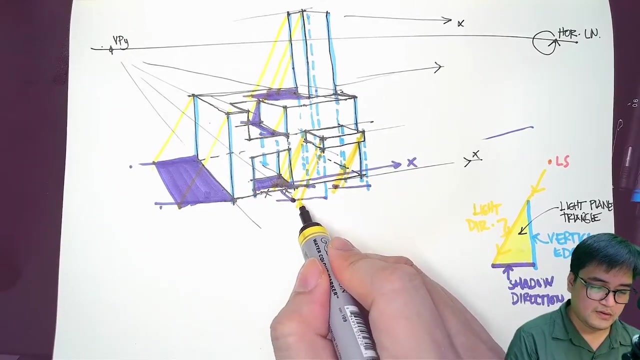 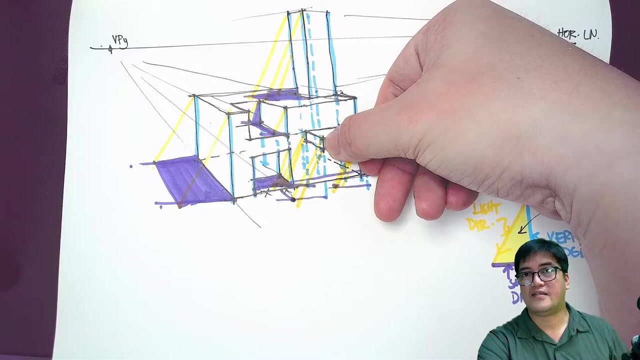 because that's how we determine and this edge is towards vanishing point Y and we follow the same edge. so it's partial. we determine those, those things first. now this one has a secondary, secondary point, for where it starts. now we could say that you know, it's the shadow, vertical, shadow edge. casting of this is 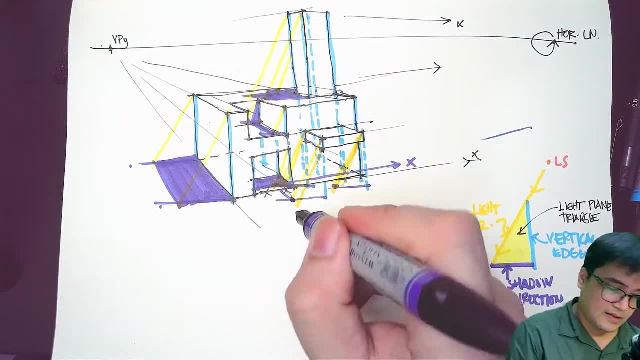 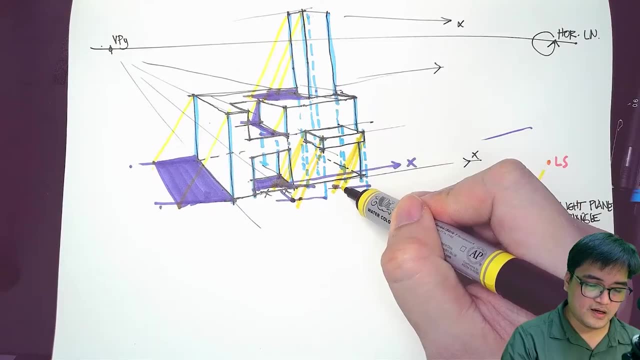 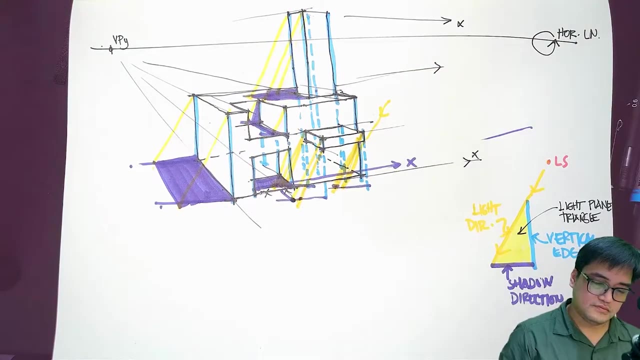 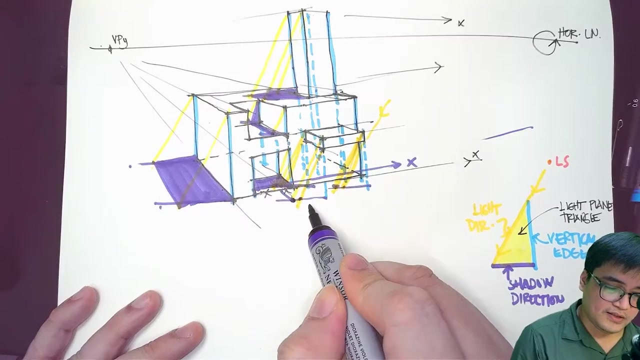 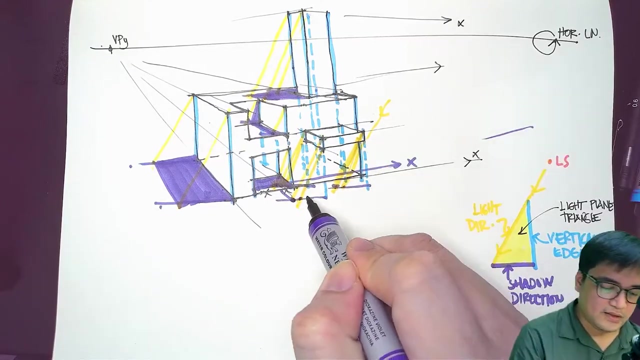 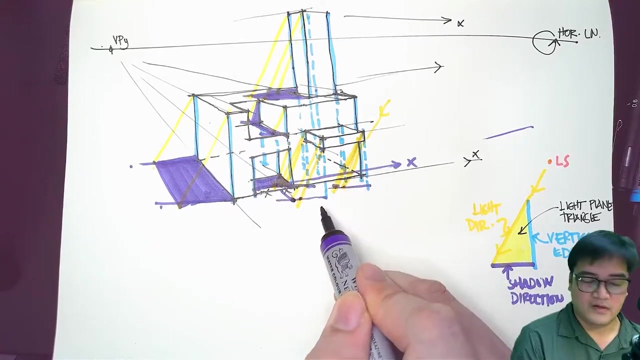 actually this up to there same way. here there's a secondary light direction and and the result is this point: now we can plot these two points on the lower casting of these vertical line shadows, and now we can determine the shadow casting of this edge, underneath this cantilever, on to here, on to the ground. 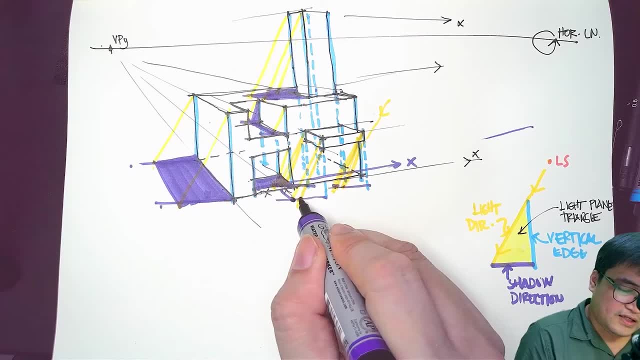 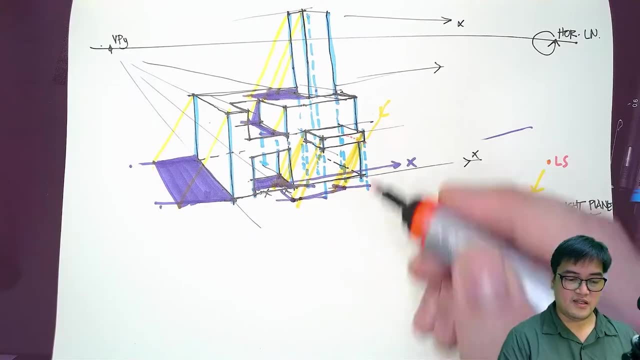 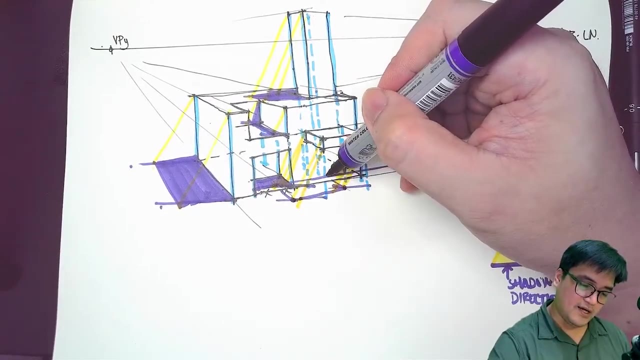 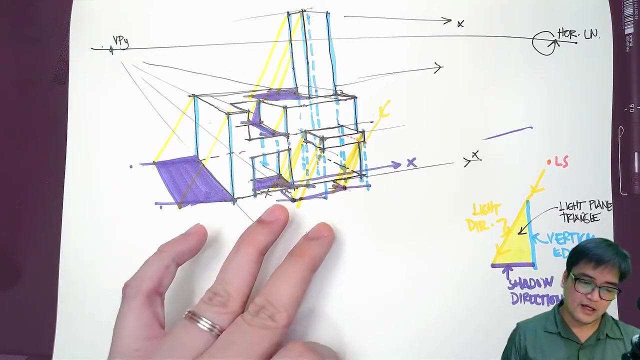 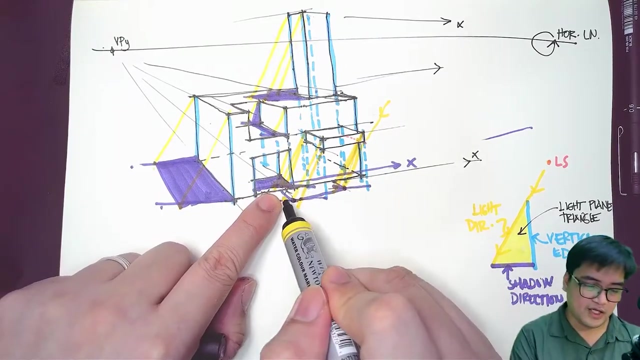 my connecting these two points underneath here on this cantilever, so we need to cast that. so from here I'm going to draw a line towards that vanishing point also. and it hits this, it hits the, the plane here under, uh, on this ground, this plane is extended, okay, so we have that line. 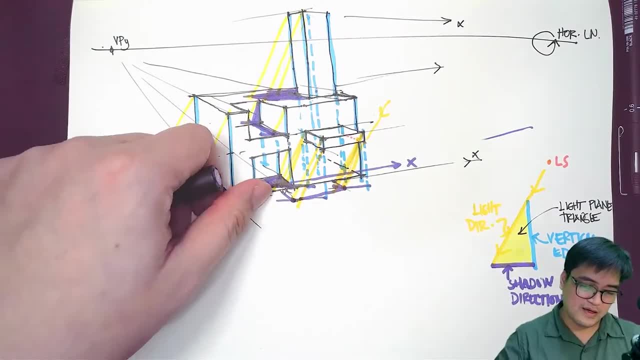 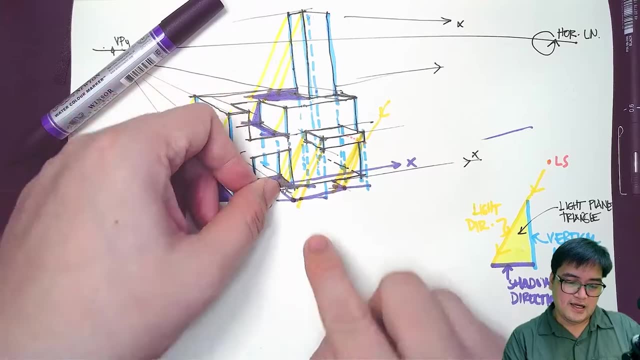 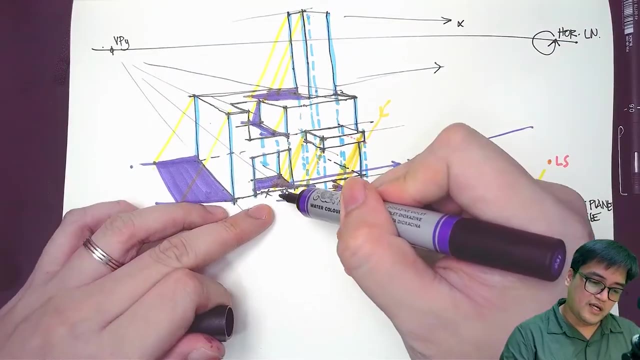 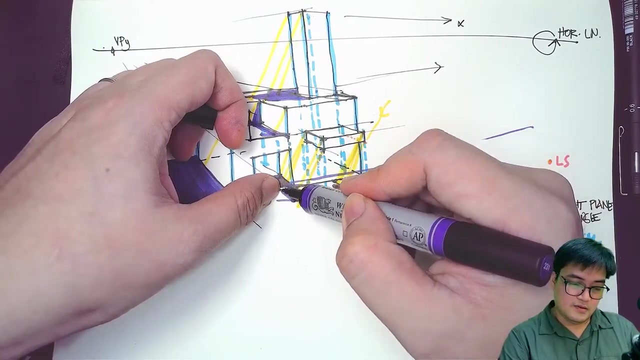 here, under uh, on this ground, this plane is extended. okay, so we have that line that determines now that intersection here, between from this point and line going towards there, intersects here. now you can illustrate from this intersection to this top, most of this line to be like. so 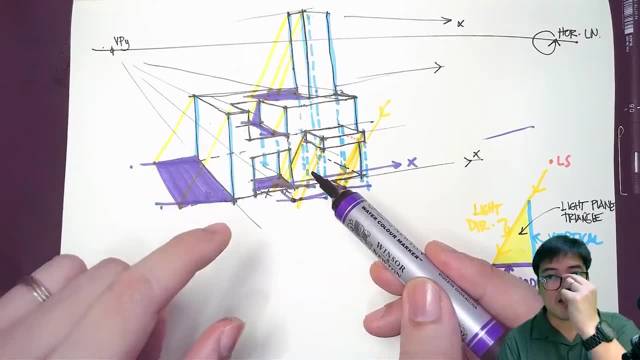 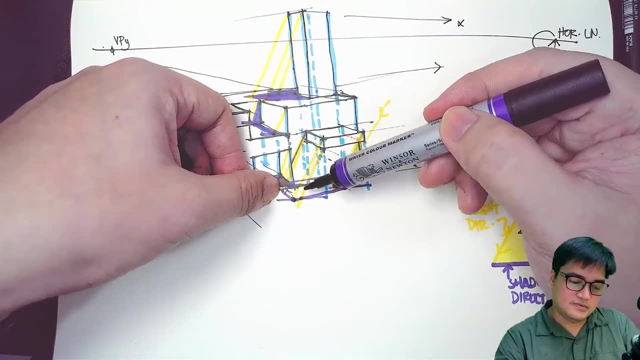 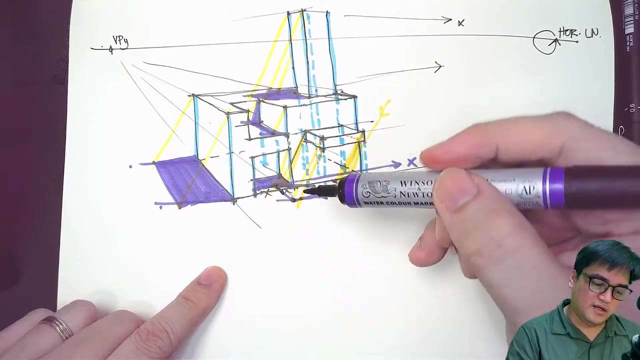 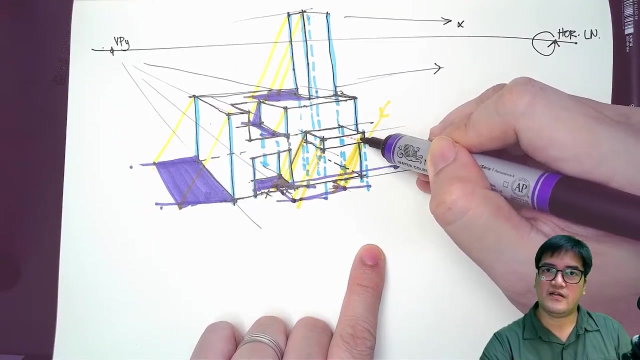 so it's a right 때는 just touching down my Negative angle side-by-side, so it's not following the light direction line and go, but rather it's from this intersection. but this shadow line distance, this, this edges shadow line, extends beyond this shadow cast, the shadow casting of this structure.